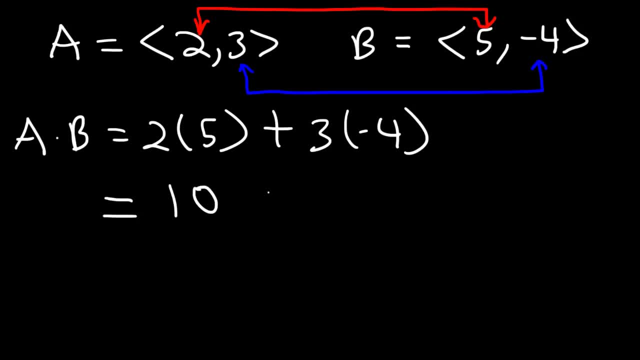 2 times 5 is 10. And 3 times negative 4 is negative 12. So it's 10 minus 12, which is negative 2. 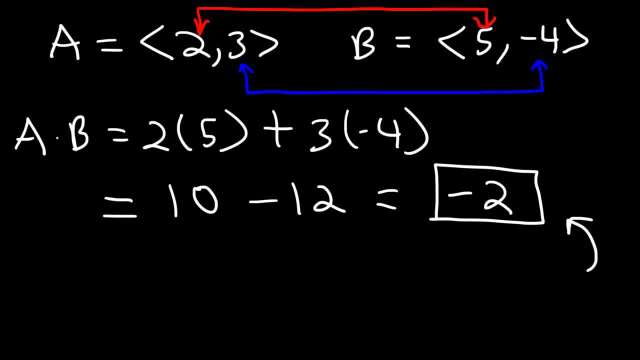 And as you can see, the answer is a scalar quantity. It's just a number. It's not a vector. 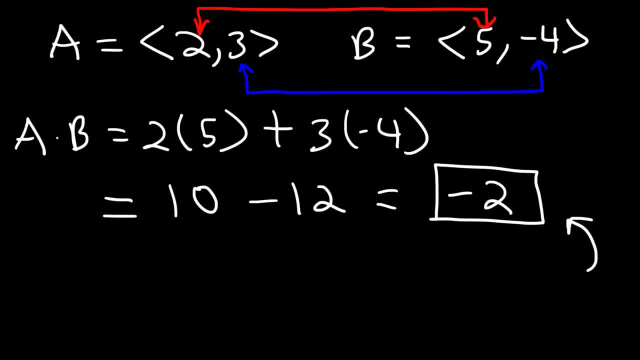 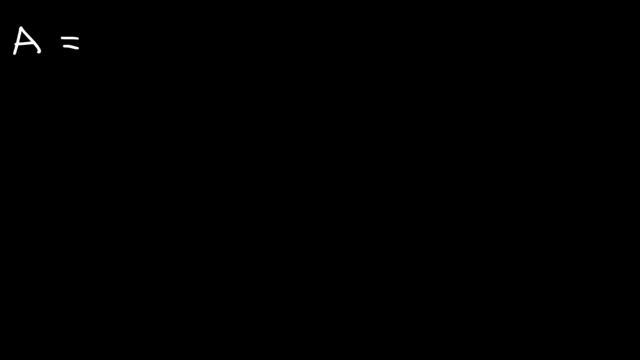 And so that's a simple way in which you could find the dot product between two vectors. Now, let's say if we have a three-dimensional vector. Let's say A is 3, negative 4, 7. 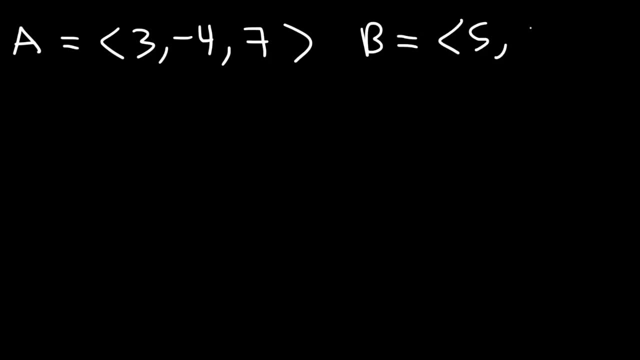 And vector B is 5, 2, negative 3. 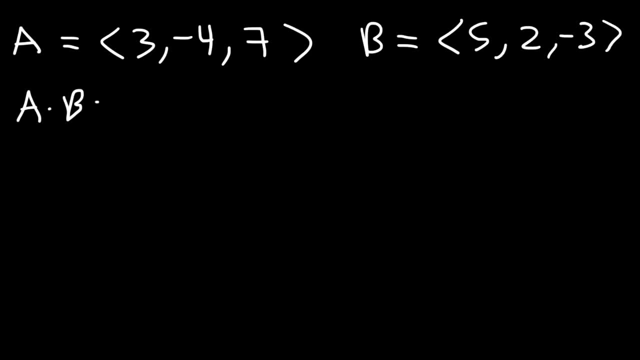 So how can we find the dot product of A and B? So if you have a three-dimensional vector, where you have the x, the y, and the z component for vectors A and B, here's the formula that you need to use. So it's going to be ax times bx. So basically, you multiply the x components together. And then plus. Multiply the y components together. 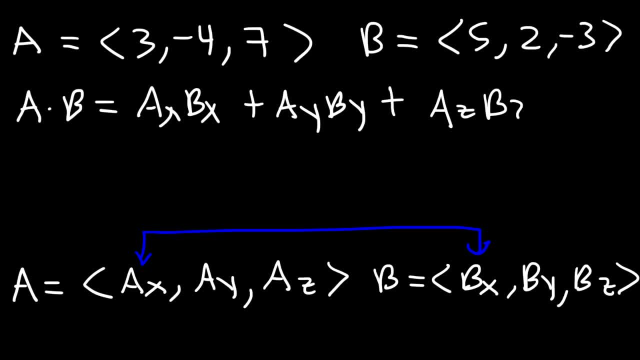 And then multiply the z components together. So that's how you could find the dot product between two vectors that have an x, y, and z component. 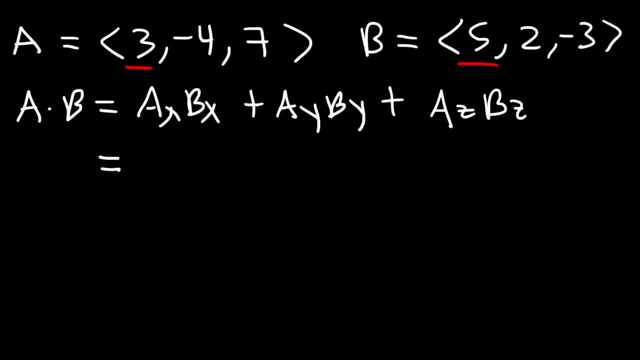 So now let's work out this example. So ax is 3, bx is 5. And then ay is negative 4. By is 2. So it's going to be negative 4 times 2. And then the z components are 7 and negative 3. 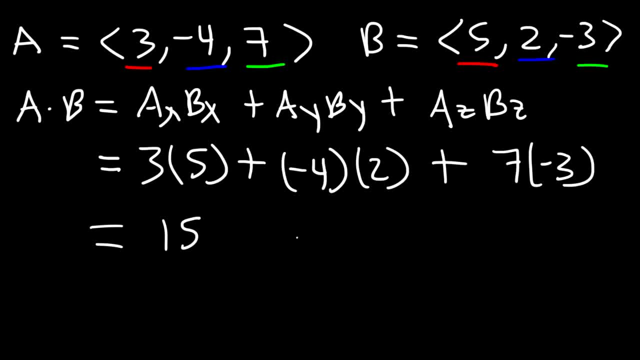 So 3 times 5, that's 15. Negative 4 times 2 is negative 8. And 7 times negative 3, that's negative 21. So 15 minus 8 is 7. 7 minus 21 is negative 14. So this is the answer for the second example. 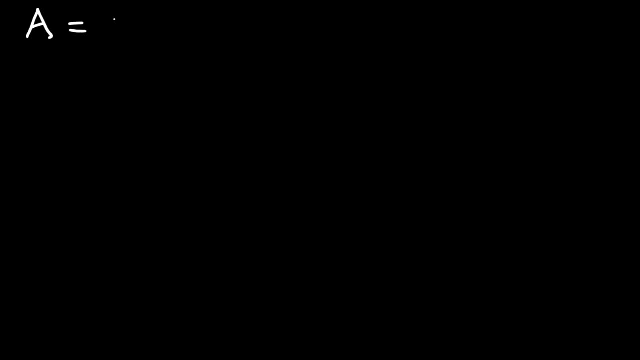 Now let's go back to our first problem where we said that vector A is 2 comma 3. And vector B is 5 comma negative 4. 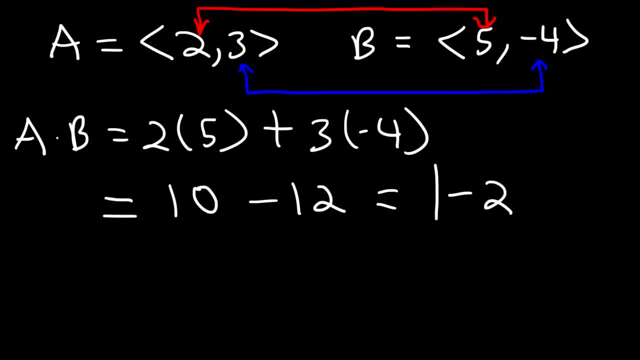 So it's 10 minus 12,, which is negative 2. And, as you can see, the answer is a scalar quantity, It's just a number, It's not a vector, And so that's a simple way in which you could find the dot product between two vectors. 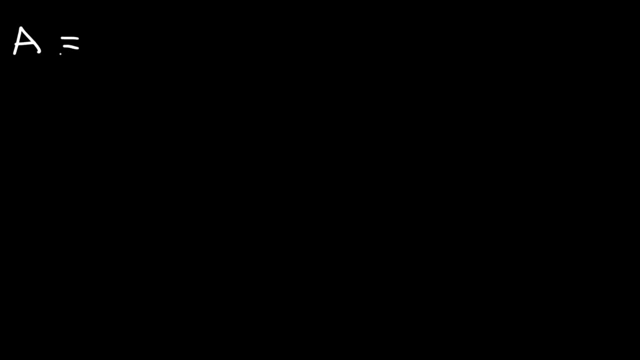 Now let's say, if we have a three-dimensional vector, Let's say A is 3, negative 4, 7. And vector B is 5, 2, negative 3. So how can we find the dot product of A and B? 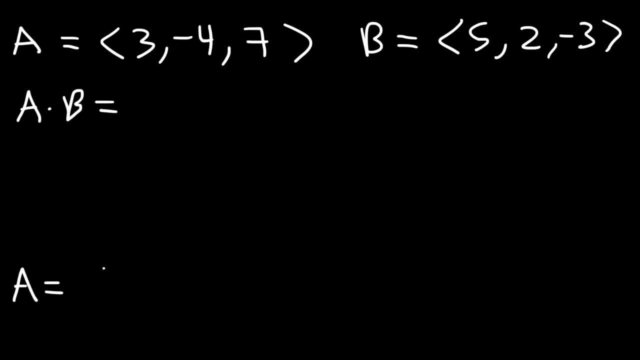 So if you have a three-dimensional vector where you have the x, the y and the z component for vectors A and B, here's the formula that you need to use. So it's going to be ax times bx. So basically, you multiply the x components together. 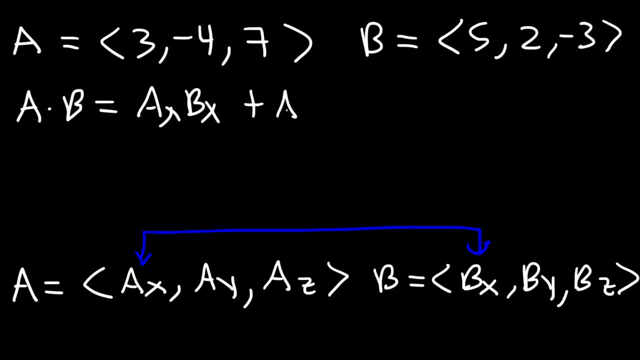 And then plus Multiply the y components together And then multiply the z components together. So that's how you could find the dot product between two vectors that have an x, y and z component. So now let's work out this example. 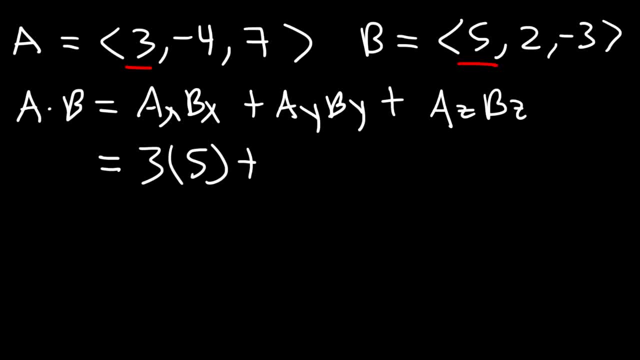 So ax is 3, bx is 5.. And then ay is negative 4.. By is 2.. So it's going to be negative 4 times 2.. And then the z components are 7 and negative 3.. So 3 times 5, that's 15.. 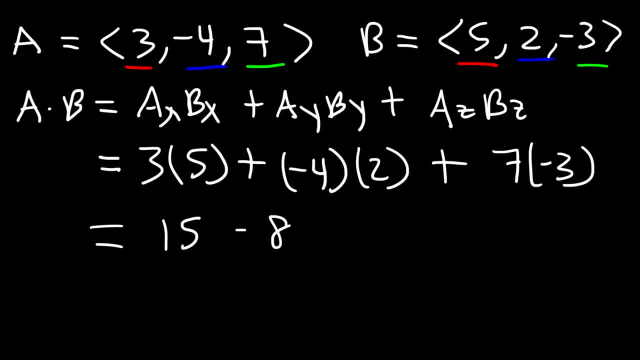 Negative. 4 times 2 is negative 8.. And 7 times negative 3, that's negative 21.. So 15 minus 8 is 7.. 7 minus 21 is negative 14.. So this is the answer for the second example. 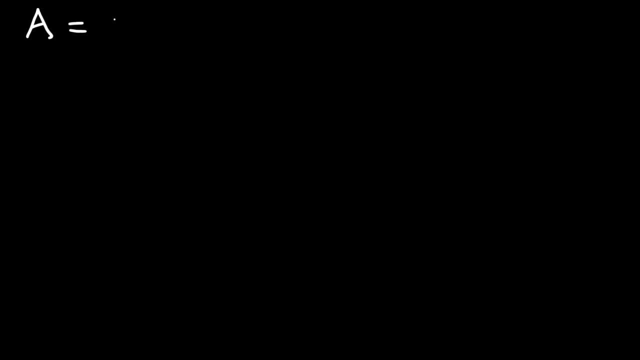 Now let's go back to our first problem, where we said that vector A is 2 comma 3.. And vector B is 5 comma negative 4.. How can we calculate the square of the magnitude of vector A? What do you think we need to do? 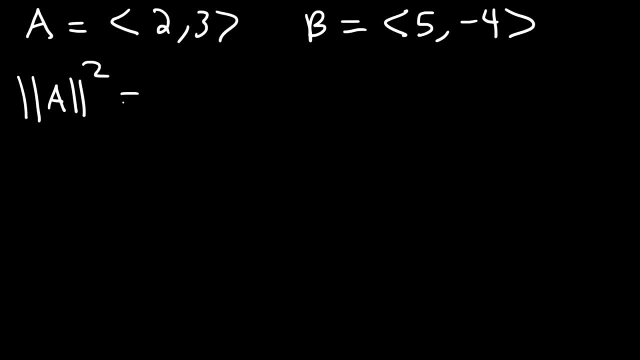 It turns out that the square of the magnitude of vector A is equal to the dot product of A and another vector A. And here is the proof for that. Now we know that to calculate the magnitude of A, it's simply equal to the square root of the square of the x component. 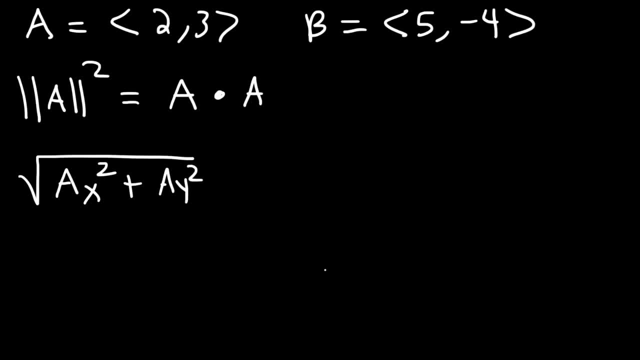 plus the square of the y component. So let's say this is the x component of vector A and this is the y component. The magnitude is the hypotenuse, The hypotenuse of the right triangle, And so it follows the Pythagorean Theorem. 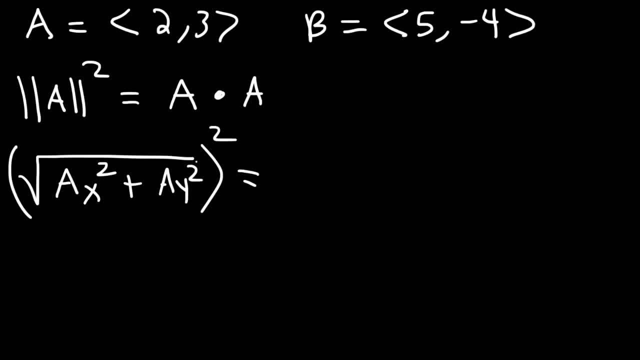 Now, because this is squared, we need to square it Now. vector A times vector A, that's going to be vector A is ax, comma, ay, multiplied by another vector A, And to perform the dot product between these two vectors we need to multiply the x components together. 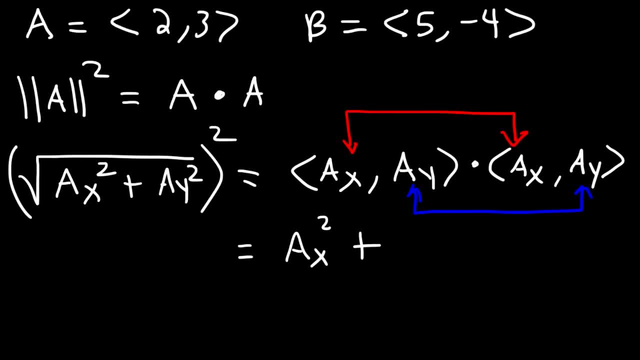 And then we need to multiply the y components together. On the left side, the square root and the square will cancel. So thus we could see that the original expression is correct. Now let's go ahead and finish the problem. So vector A is 2 comma 3.. 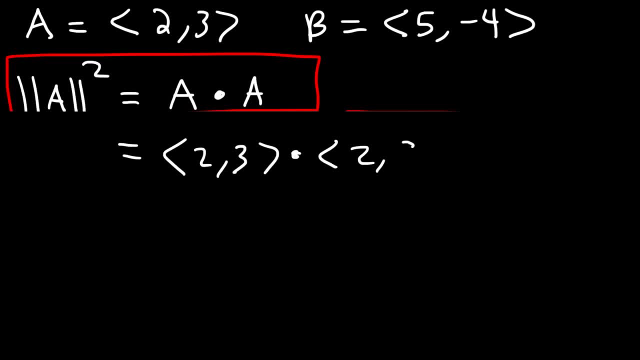 And let's multiply it by another vector, A, So we're going to multiply 2 by 2. And so that's equal to 4.. And then we're going to multiply 3 by 3, which is 9.. So the answer for this example is 13.. 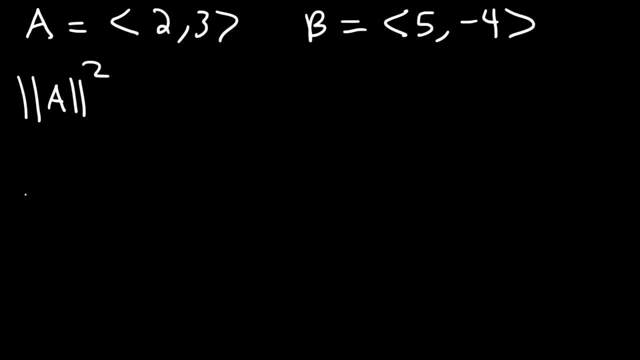 How can we calculate the square of the magnitude of vector A? What do you think we need to do? 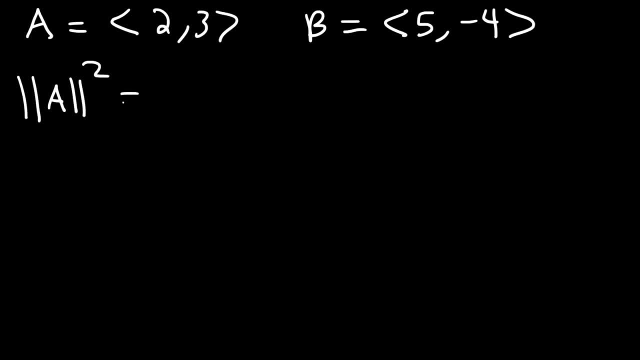 It turns out that the square of the magnitude of vector A is equal to the dot product of A and another vector A. And here is the proof for that. 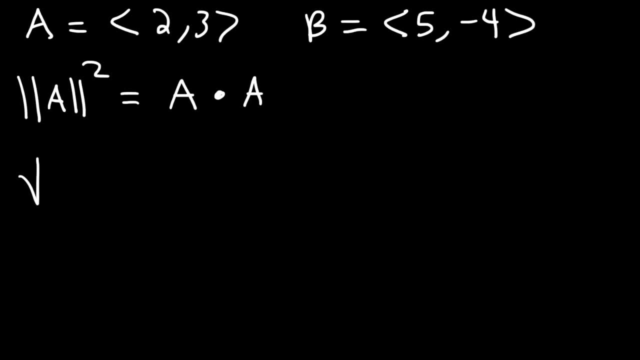 Now we know that to calculate the magnitude of A, it's simply equal to the square root of the square of the x component plus the square of the y component. 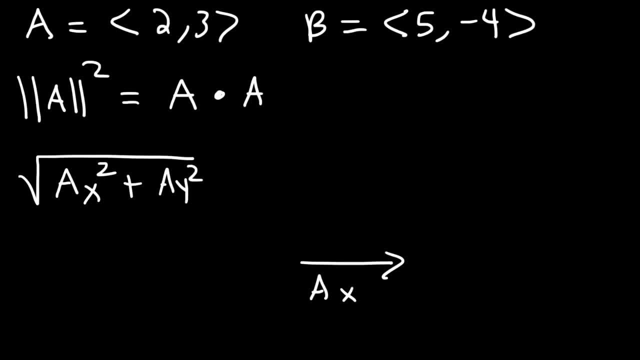 So let's say this is the x component of vector A and this is the y component. 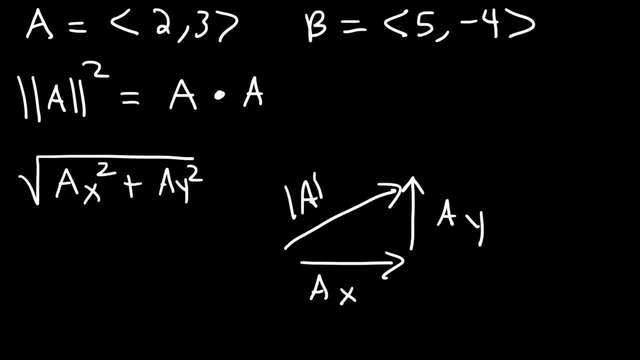 The magnitude is the hypotenuse. The hypotenuse of the right triangle. 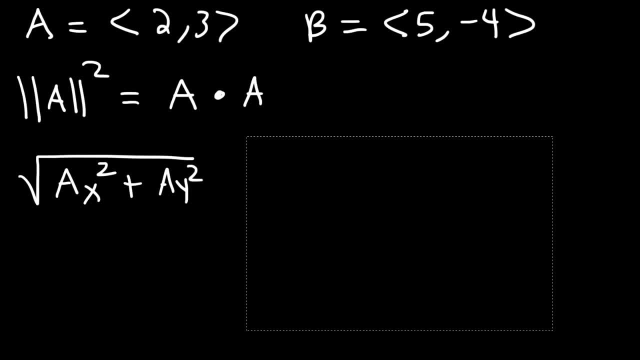 And so it follows the Pythagorean Theorem. Now because this is squared, we need to square it. 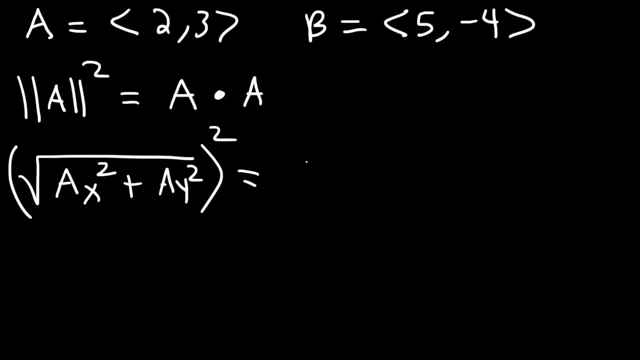 Now vector A times vector A, that's going to be vector A is ax comma ay multiplied by another vector A. 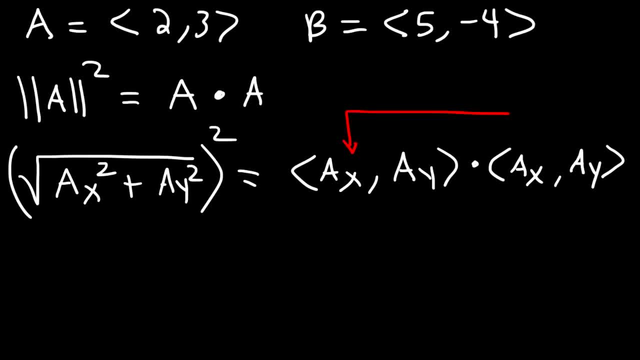 And to perform the dot product between these two vectors, we need to multiply the x components together. 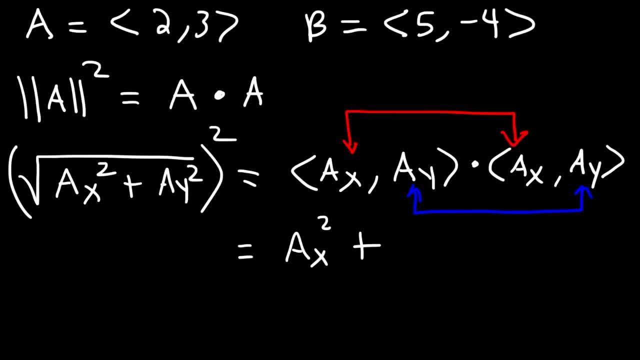 And then we need to multiply the y components together. 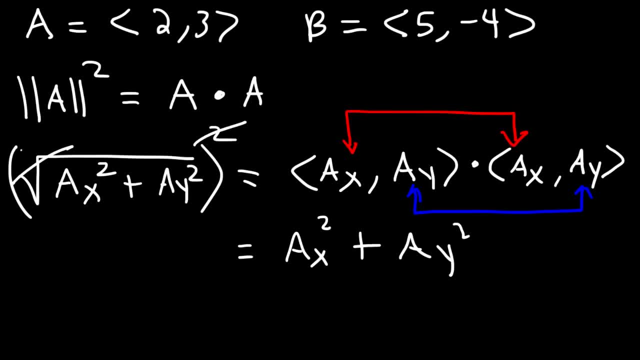 On the left side, the square root and the square will cancel. So thus we could see that the original expression is correct. 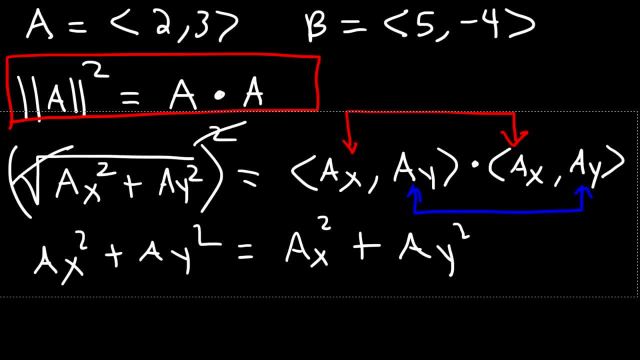 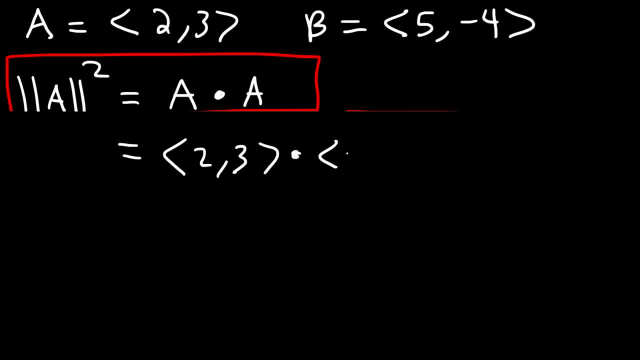 Now let's go ahead and finish the problem. So vector A is 2 comma 3. And let's multiply it by another vector A. So we're going to multiply 2 by 2. And so that's equal to 4. And then we're going to multiply 3 by 3, which is 9. So the answer for this example is 13. Now here's another problem that you can work on. 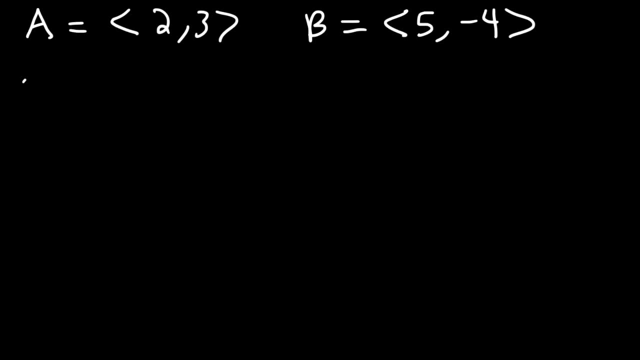 Now here's another problem that you can work on: Calculate the dot product of A and B times vector A. Go ahead and try that. So we have vector A, which is 2 comma 3.. And then vector B, which is 5 negative 4.. 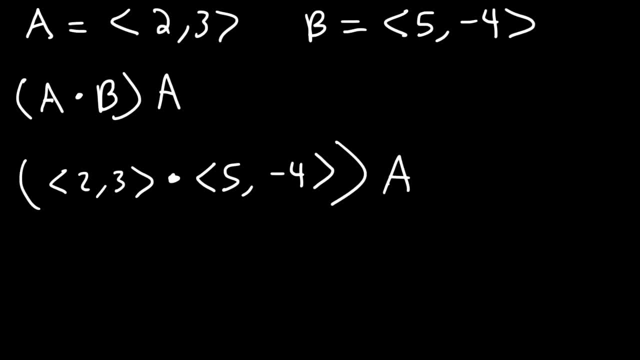 And then, whatever result we get from that, we're going to multiply it by vector A, Which is 2, 3.. So this is going to be 2 times 5,, which is 10. And then 3 times negative 4.. 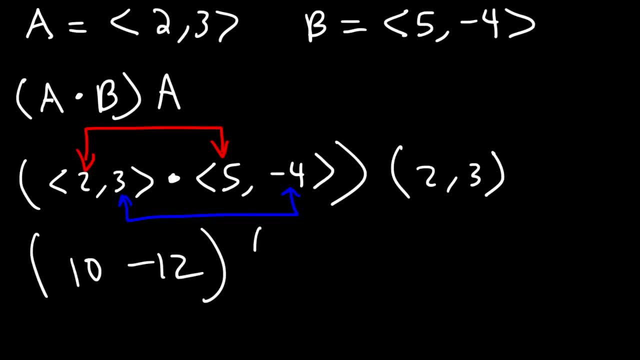 So that's negative 12.. And then times? Well, this is a vector, so I need to put this in. I need to use inequality symbols as opposed to parentheses. Now, 10 minus 12 is negative 2.. So what I'm doing is I'm multiplying vector A by 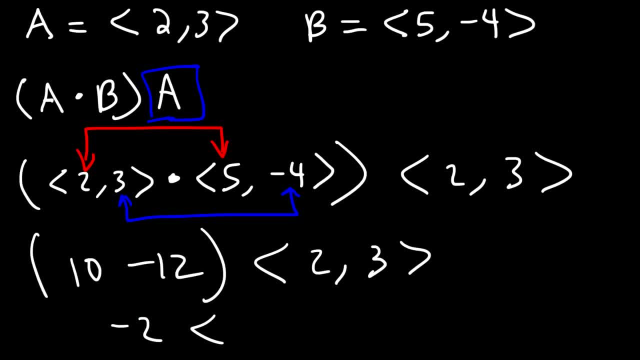 Here's vector A. I'm multiplying it by negative 2.. So it's going to be negative 2 times 2,, which is negative 4.. And then negative 2 times 3,, which is negative 6.. So this result: 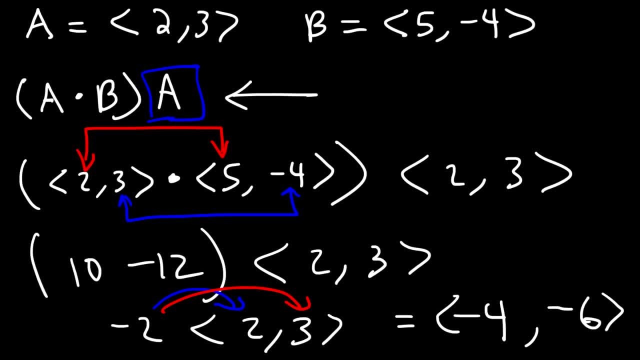 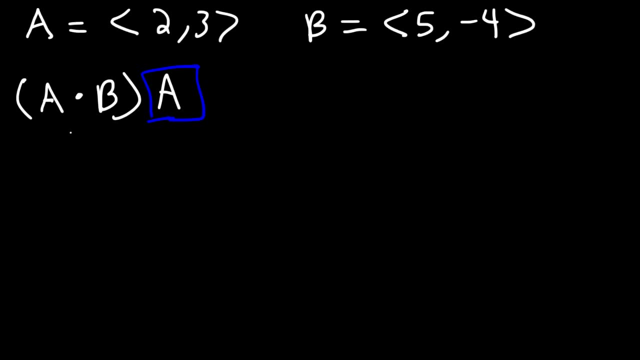 gives us a vector and not a scalar quantity. Now, for those of you who might be a little confused on exactly what just happened here, let me just review what's going on. So once we calculated the dot product between A and B, we got a scalar quantity which was negative 2.. 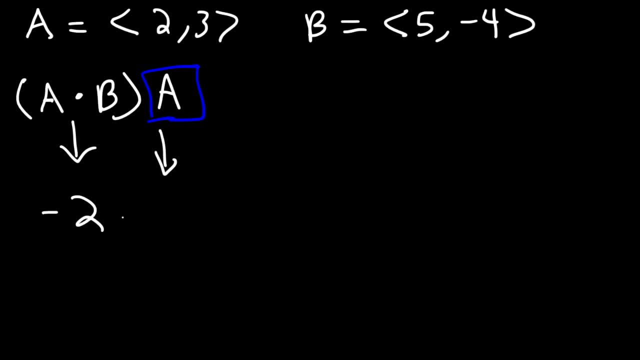 Now, when you multiply a vector by a scalar quantity, you still get another vector, which is what we did at the end, And that gave us the vector negative 4,, negative 6.. And so make sure you understand that. So the dot product gives you a scalar quantity. 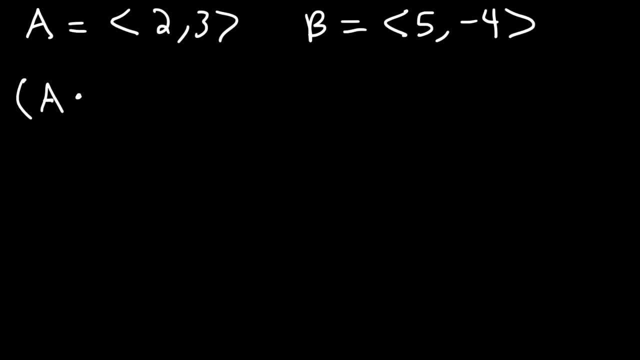 Calculate the dot product of A and B times vector A. Go ahead and try that. So we have vector A, which is 2 comma 3. And then vector B, which is 5 negative 4. And then whatever result we get from that, we're going to multiply it by vector A. 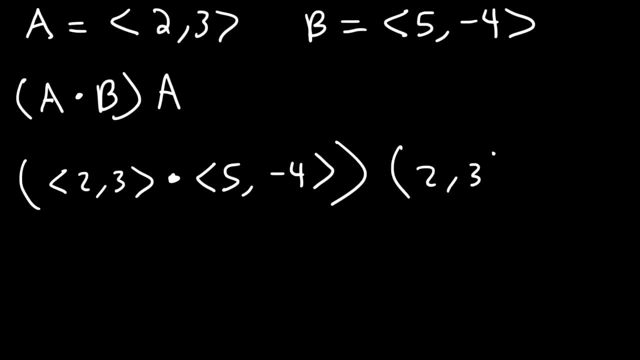 Which is... 2, 3. 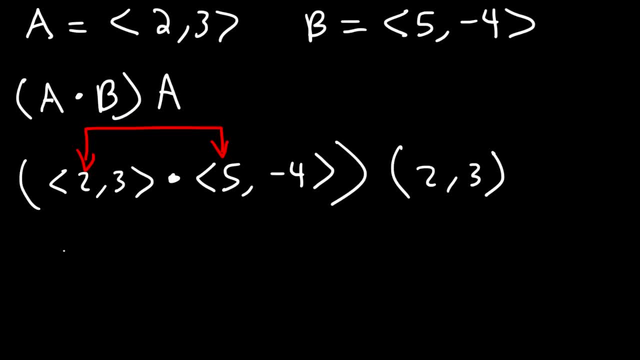 So this is going to be 2 times 5, which is 10. 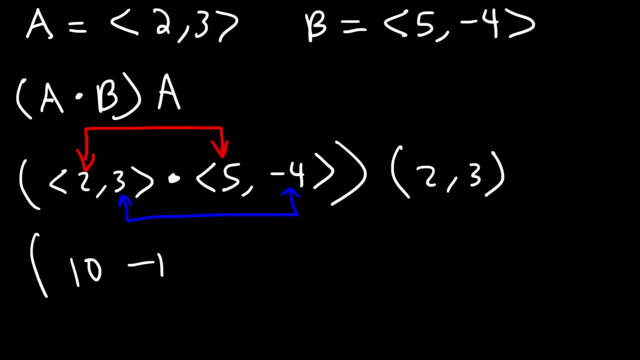 And then 3 times negative 4. So that's negative 12. 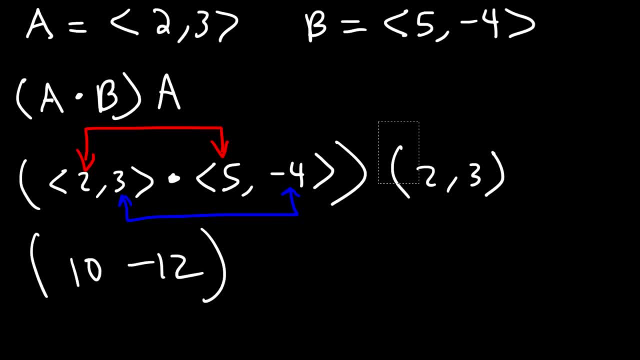 And then times... Well this is a vector, so I need to put this in... I need to use inequality symbols as opposed to parentheses. 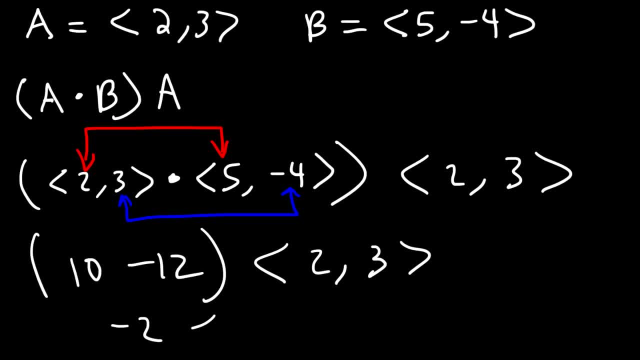 Now 10 minus 12 is negative 2. So what I'm doing is I'm multiplying vector A by... Here's vector A. I'm multiplying it by negative 2. 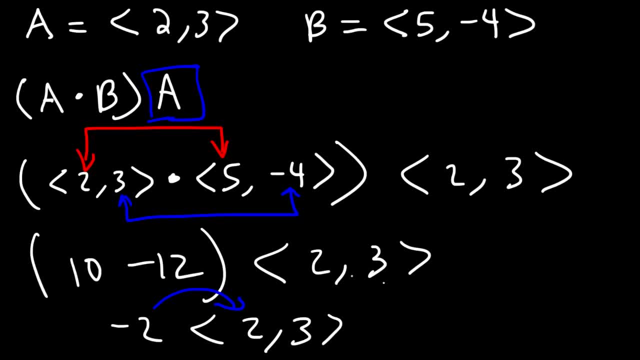 So it's going to be negative 2 times 2, which is negative 4. 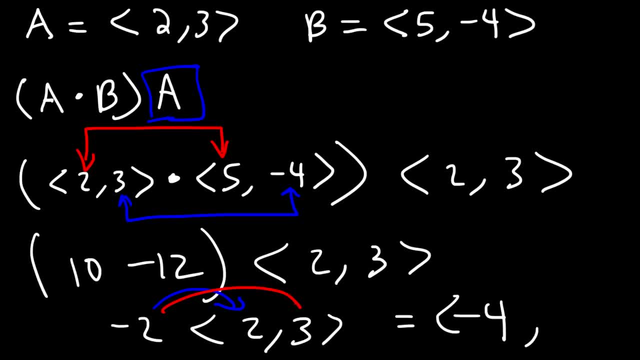 And then negative 2 times 3, which is negative 6. 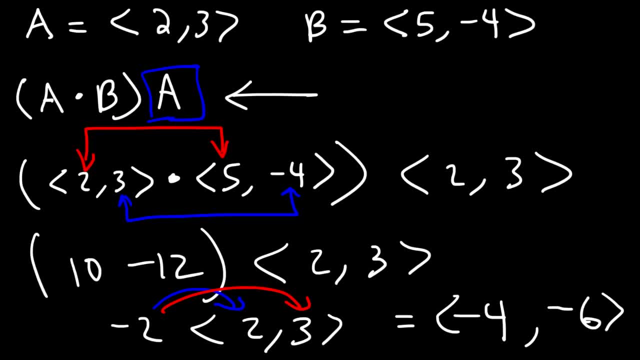 So this result... gives us a vector and not a scalar quantity. 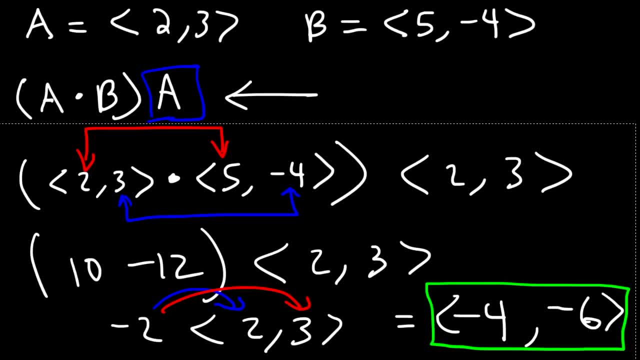 Now for those of you who might be a little confused on exactly what just happened here, let me just review what's going on. 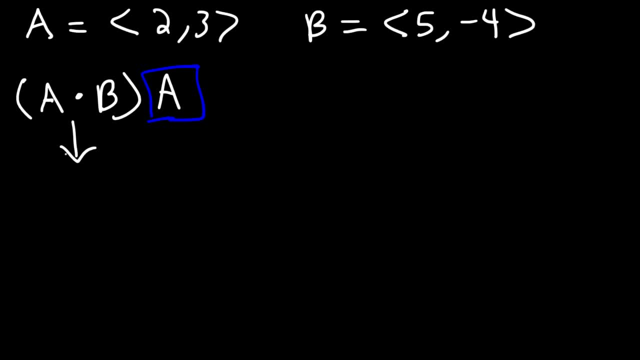 So once we calculated the dot product between A and B, 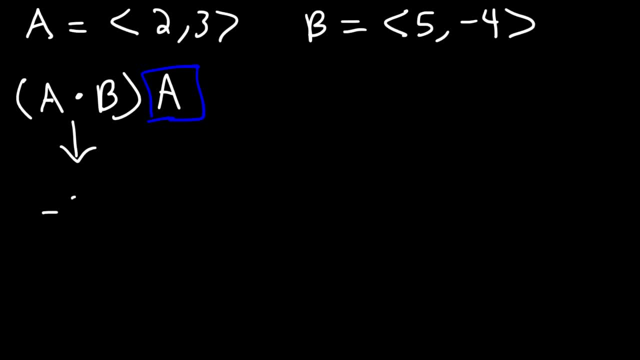 we got a scalar quantity, which was negative 2. Now when you multiply a vector by a scalar quantity, you still get another vector, which is what we did at the end. 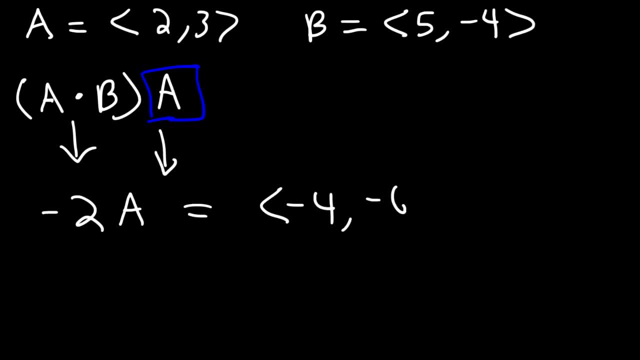 And that gave us the vector negative 4, negative 6. And so make sure you understand that. 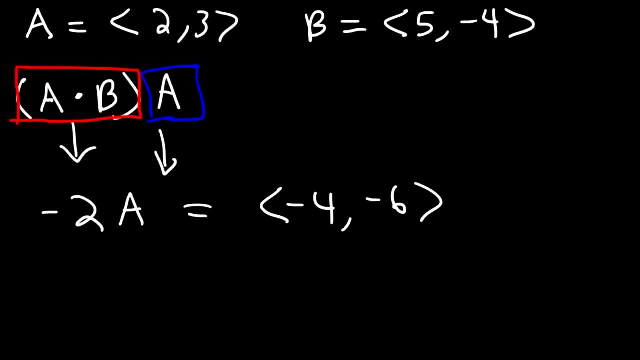 So the dot product gives you a scalar quantity, and whenever you multiply a scalar by a vector, you get another vector. 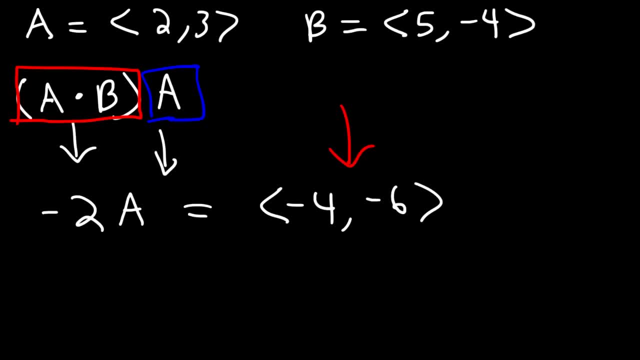 and whenever you multiply a scalar by a vector, you get another vector. Let's try a different example. Calculate the dot product between B and 3A, So will this expression, will the answer to this expression be a scalar quantity or a vector quantity? 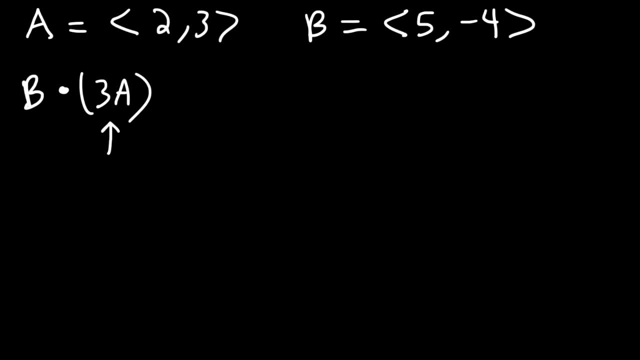 What would you say Now? 3 times A, a scalar times vector A will give us a vector quantity And then once we take that vector and find the dot product between another vector, that's going to give us a scalar result. So in the end we should get: 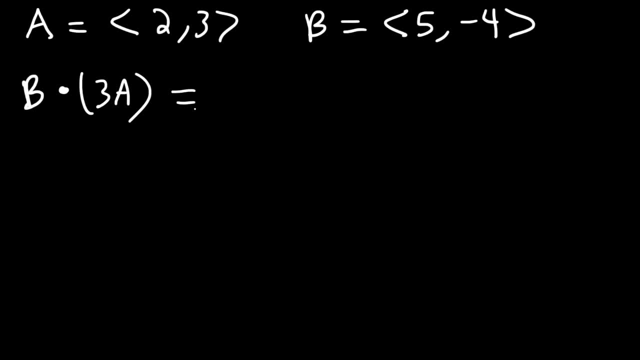 just a number. So vector B is 5, negative 4, and then we're going to multiply vector A by 3.. So let's do that first. So 3 times 2 is 6, and then we have 3 times 3,, which is 9.. 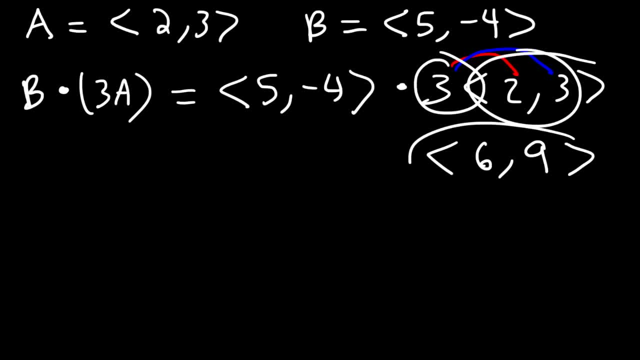 So a scalar times a vector gives you another vector. So now we're going to take the dot product between two vectors and that's going to give us a scalar result. So first we're going to multiply 5 times 6, which is 30,. 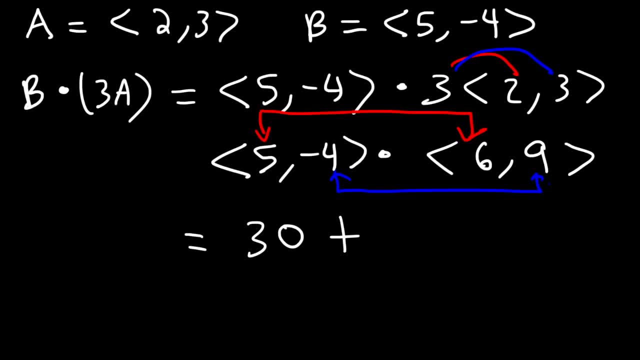 and then we're going to multiply negative 4 times 9,, which is negative 36.. And 30 minus 36 is negative 6.. So that's the scalar result of the dot product between vector B and 3 times vector A. 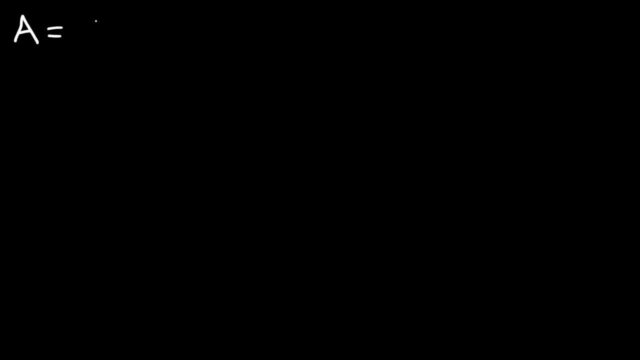 Now let's try another problem. Let's say vector A is 4, 5, and vector B is 3, negative 6, and vector C is negative 8, 2. Go ahead and calculate the dot product between vector A and the sum. 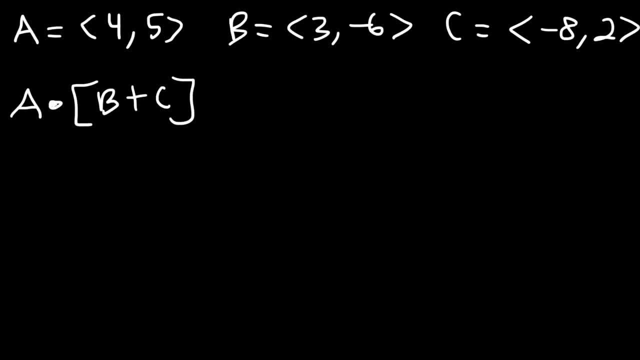 of vectors B and C. Go ahead and try that. So vector A is 4, 5, and then we need to multiply that by B plus C. So that's vector B, and here is vector C. So the first thing we're going to do, 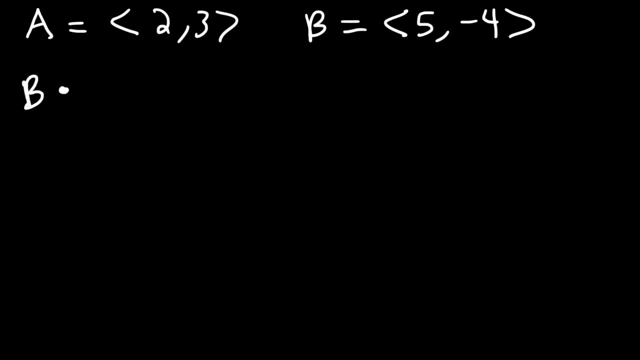 Let's try a different example. Calculate the dot product between B and 3A. 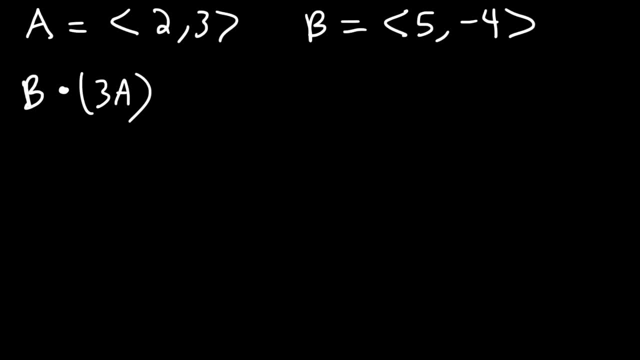 So will this expression... will the answer to this expression be a scalar quantity or a vector quantity? 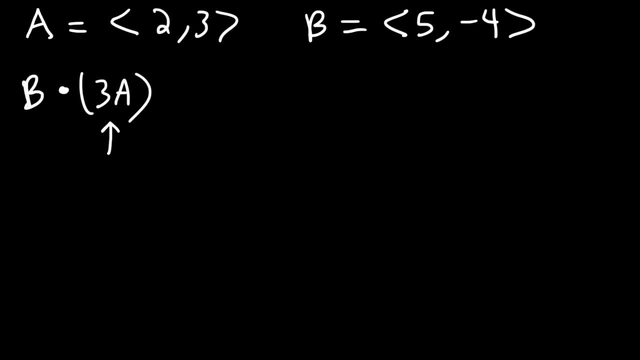 What would you say? Now 3 times A, a scalar times vector A will give us a vector quantity. 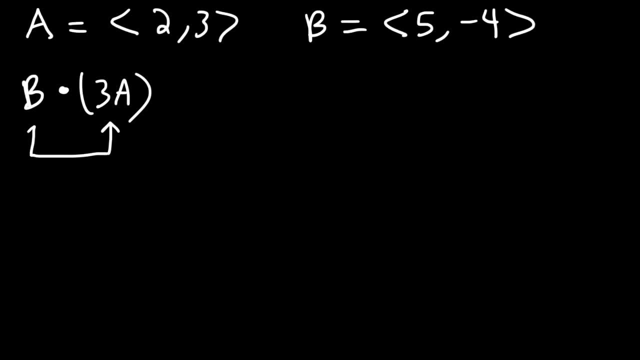 And then once we take that vector and find the dot product between another vector, that's going to give us a scalar result. 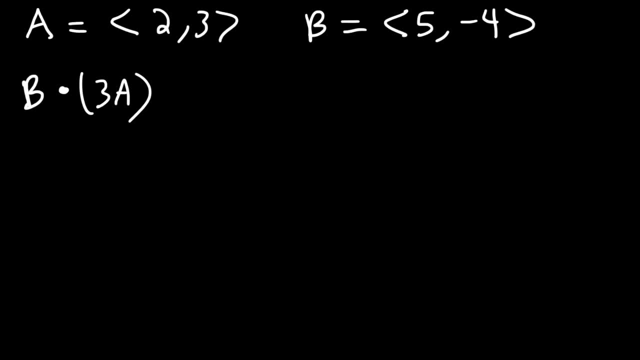 So in the end, we should get just a number. 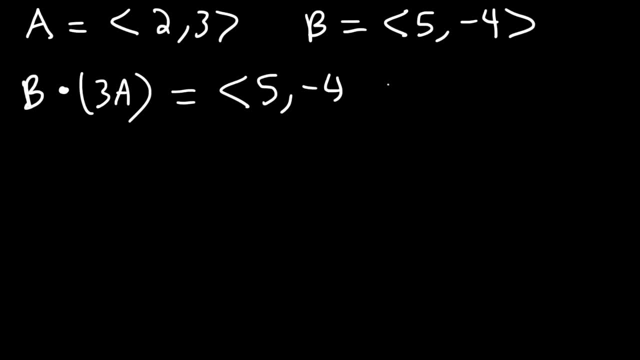 So vector B is 5, negative 4, and then we're going to multiply vector A by 3. So let's do that first. 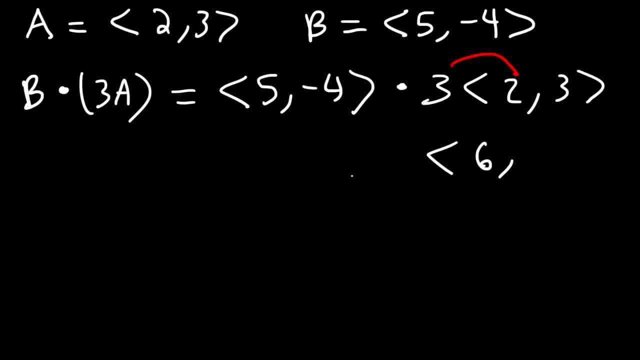 So 3 times 2 is 6, and then we have 3 times 3, which is 9. So a scalar times a vector gives you another vector. 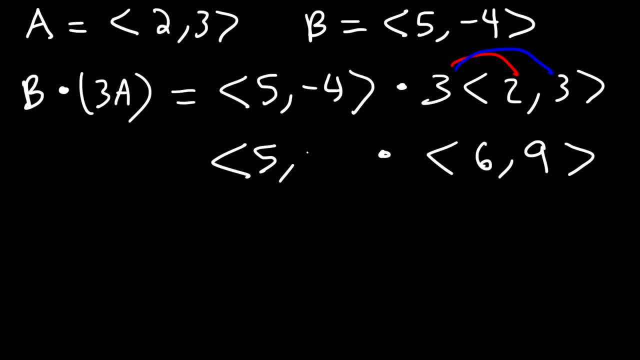 So now we're going to take the dot product between two vectors, and that's going to give us a scalar result. 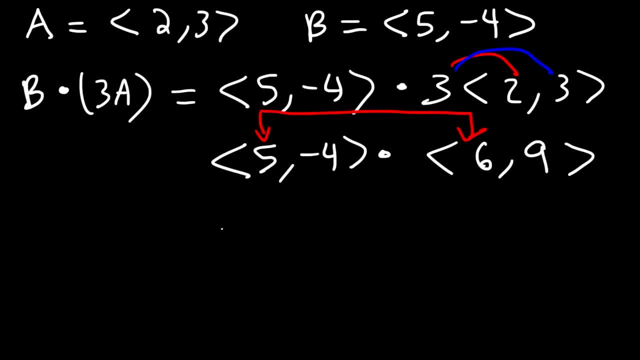 So first we're going to multiply 5 times 6, which is 30, and then we're going to multiply negative 4 times 9, which is negative 36. 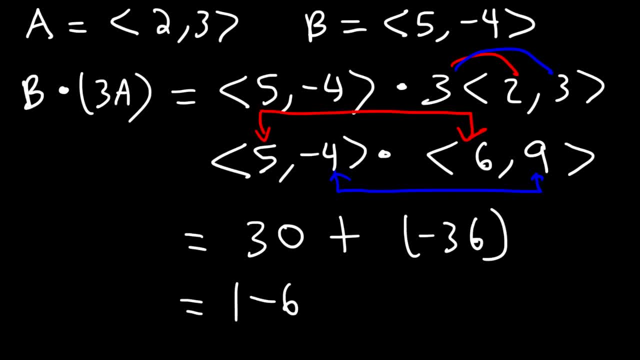 And 30 minus 36 is negative 6. So that's the scalar result of the dot product between vector B 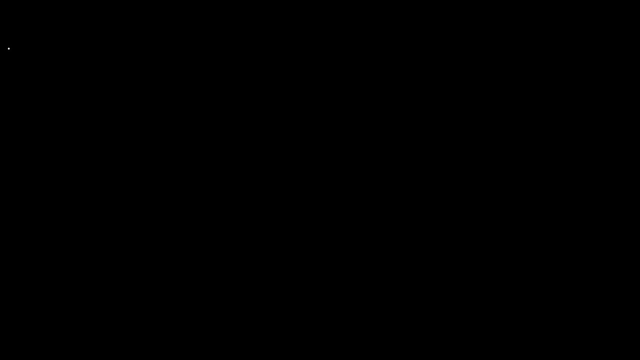 and 3 times vector A. Now let's try another problem. 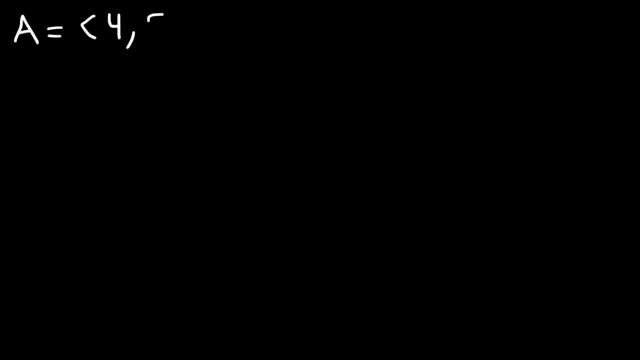 Let's say vector A is 4, 5, and vector B is 3, negative 6, and vector C is negative 8, 2. 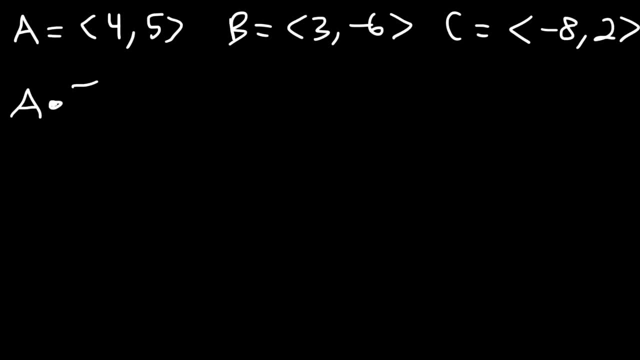 Go ahead and calculate the dot product between vector A and the sum of vectors B and C. Go ahead and try that. 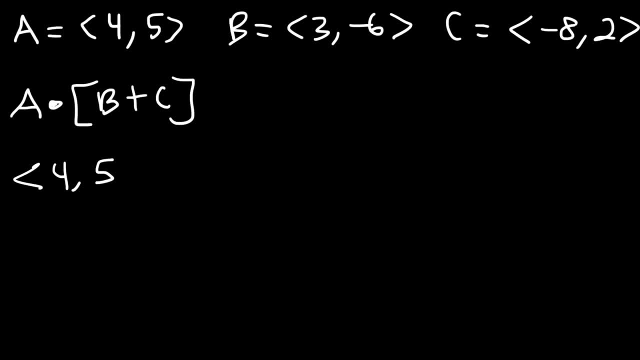 So vector A is 4, 5, and then we need to multiply that by B plus C. So that's vector B, and here is vector C. So the first thing we're going to do is add the two vectors. When you're adding vectors, you need to add the corresponding components. 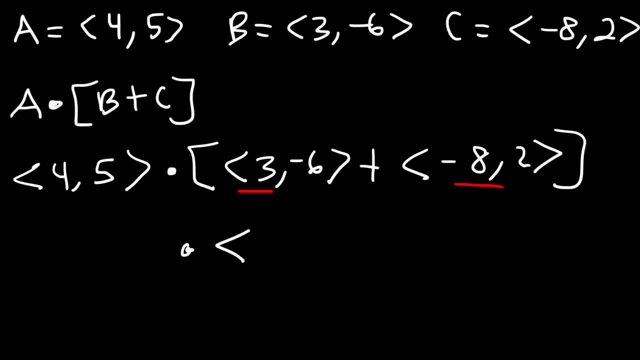 So first we have 3 plus negative 8, which is negative 5, and then we need to add the y components. Negative 6 plus 2 is negative 4. So that's the sum of vectors B and C. 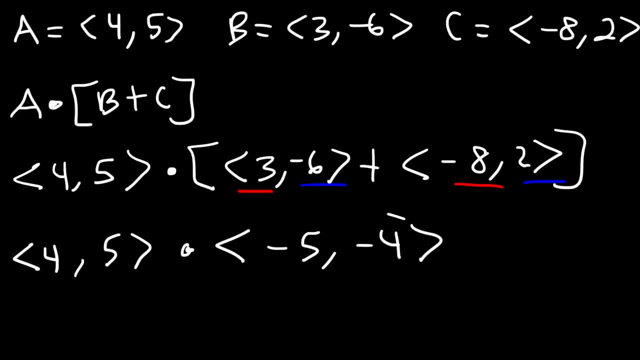 Now let's find the dot product between this vector and vector A. So first we need to multiply the x components together. 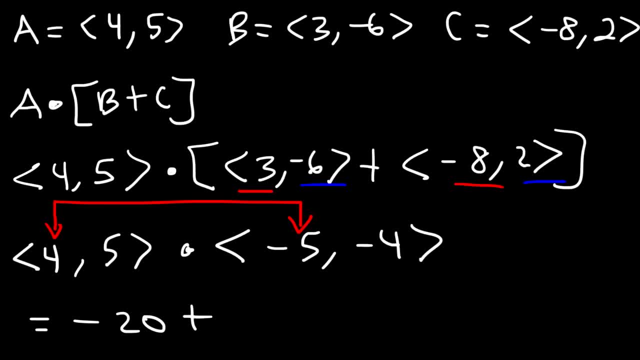 4 times negative 5 is negative 20. And then we need to multiply the y components. 5 times negative 4 is also negative 20, and so this adds up to negative 40. Therefore, this is the answer. 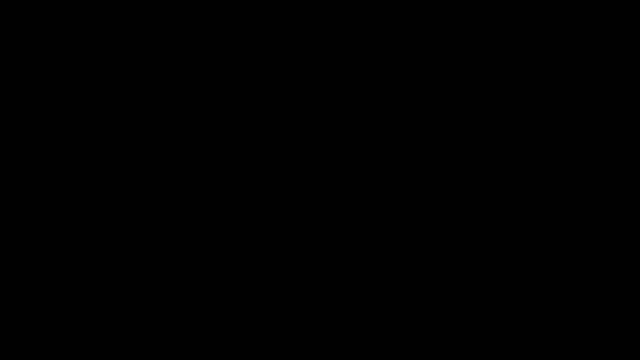 Now let's work on one more question. So let's say if we have the magnitude of vector A, and it's equal to 15, and we also have the magnitude of vector B, which is 10, and we have the angle between the two vectors, which we'll say is 30 degrees. 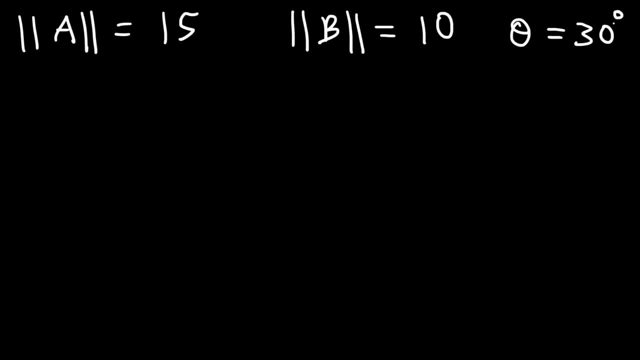 With this information, how can we calculate the dot product of A and B? 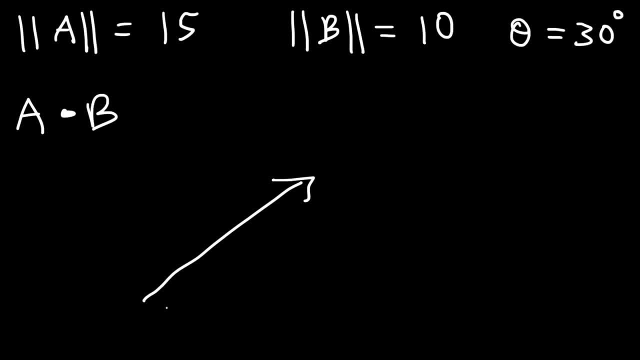 So imagine if this is vector A, and let's say this is vector B. It has to be shorter. And we have the angle between them, which is 30 degrees. 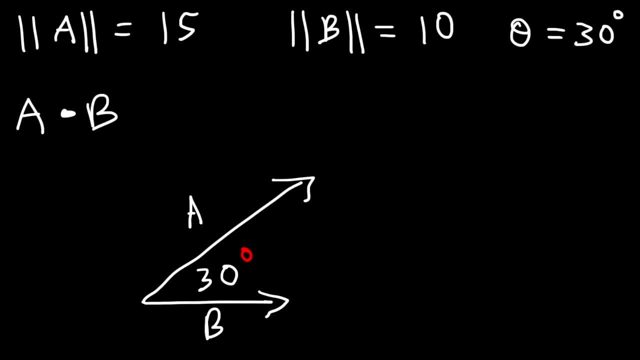 With this information, how can we calculate the dot product of the two vectors? Now there is a simple formula that we need to use. 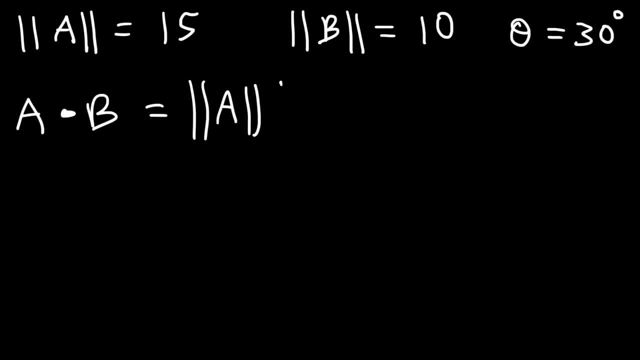 And it's the product of the magnitudes A times B, multiplied by the cosine of the angle between them. 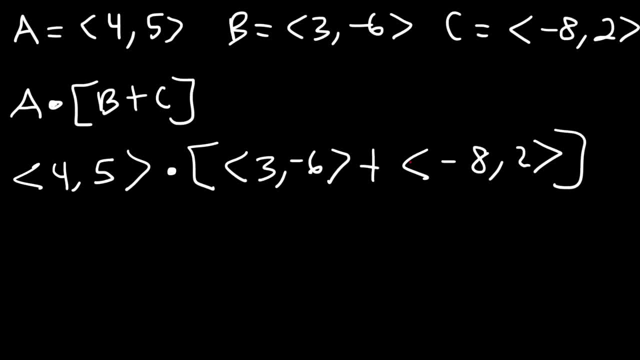 is, add the two vectors. When you're adding vectors, you need to add the corresponding components. So first we have 3 plus negative 8, which is negative 5, and then we need to add the y components. Negative 6 plus 2 is negative 4.. 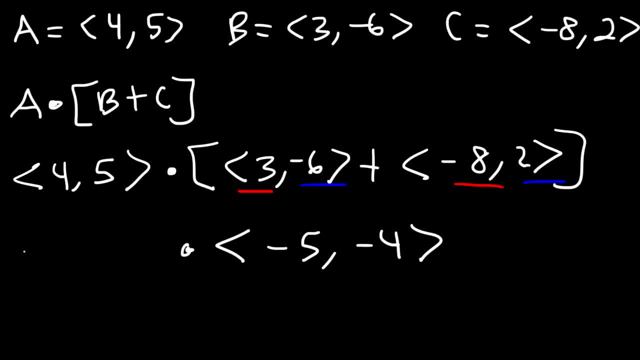 So that's the sum of vectors B and C. Now let's find the dot product between this vector and vector A. So first we need to multiply the x components together 4 times negative 5 is negative 20.. And then we need to. 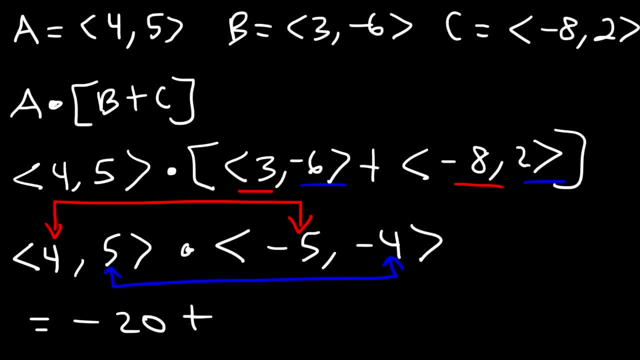 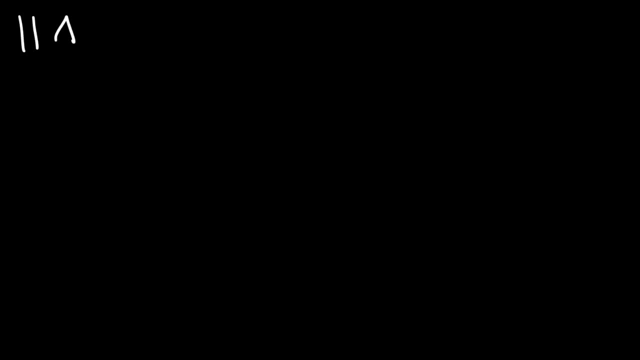 multiply the y components 5 times negative 4 is also negative 20, and so this adds up to negative 40. Therefore, this is the answer. Now let's work on one more question. So let's say if we have the magnitude, 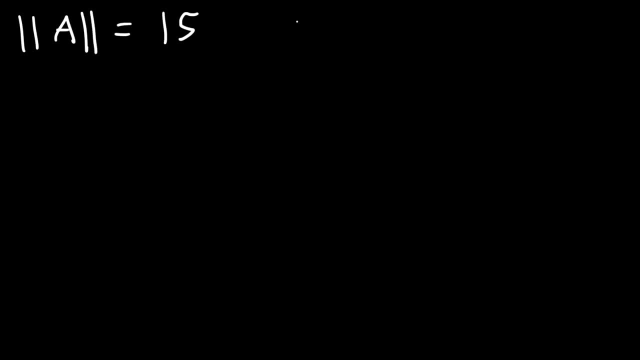 of vector A, and it's equal to 15, and we also have the magnitude of vector B, which is 10, and we have the angle between the two vectors, which we'll say is 30 degrees. With this information, how can we calculate the dot product? 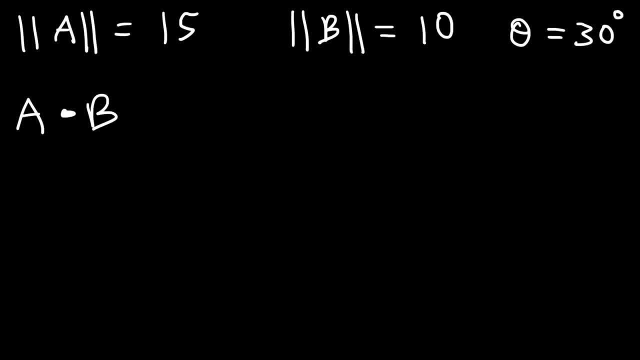 of A and B. So imagine if this is vector A and let's say this is vector B. It has to be shorter And we have the angle between them, which is 30 degrees. With this information, how can we calculate the dot product? 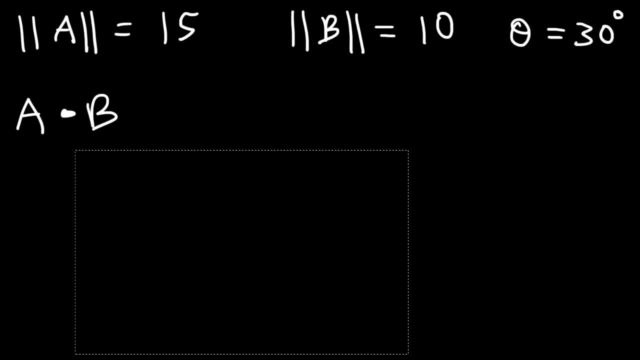 of the two vectors. Now there is a simple formula that we need to use, And it's the product of the magnitudes A times B, multiplied by the cosine of the angle between them. So the magnitude of vector A is 15, and the magnitude of vector B is 10,. 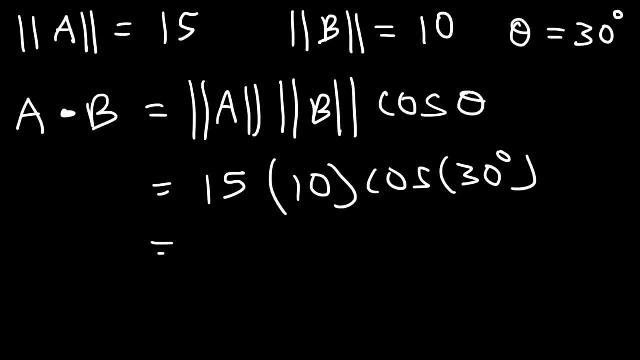 times cosine of 30 degrees. Now, 15 times 10 is 150, and cosine 30 is equal to the square root of 3 over 2.. So 150 divided by 2 is 75.. So the dot product of A and B.